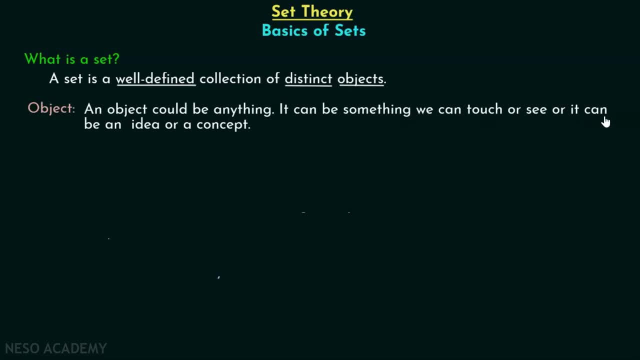 anything. let me tell you, It can be something we can touch or see, or it can be an idea or a concept. Fine, So here are some examples which help you to understand what is an object? A set of all facts learned in a discrete mathematics course. Here, facts are objects. A collection of pens, a collection. 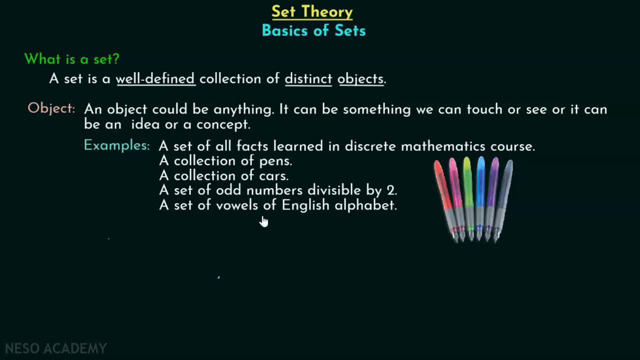 of cars, a set of odd numbers divisible by two, a set of vowels of English alphabet: Pens, cars, odd numbers divisible by two vowels, facts, these are all objects. But what is not a set? A collection of beautiful songs is not set. What, But why? Why? this is not a set. This is where the 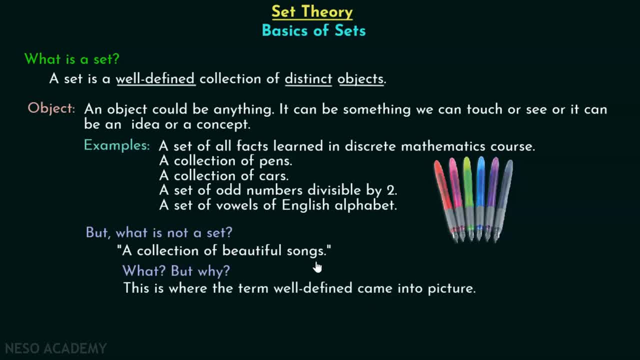 term well-defined came into picture In order to understand this, why this is not a set- we must understand the term well-defined properly. A set is considered to be well-defined if it is possible to establish that any given object belongs to the set. Okay, 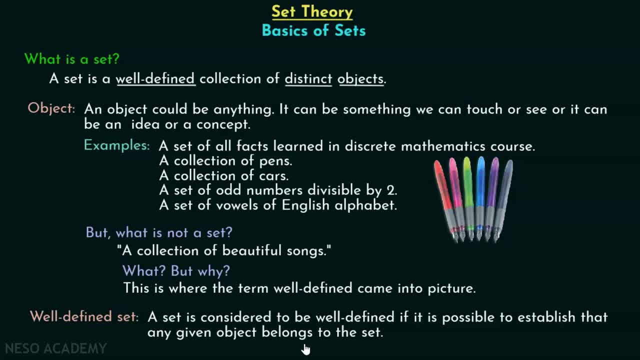 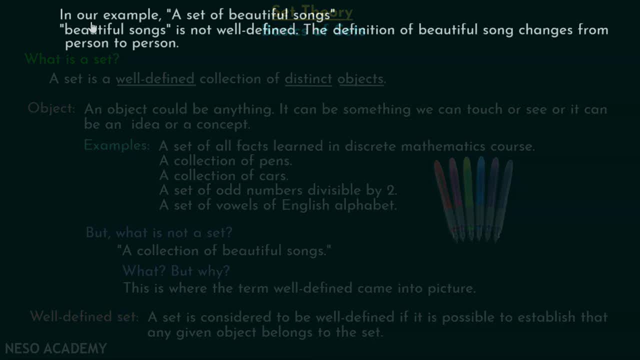 When it is possible to establish this fact, that any given object belongs to the set, then you can say that a set is well-defined. Let's just try to understand this properly with the help of an example. In our example, a set of beautiful songs- beautiful songs- is not well-defined. let me tell. 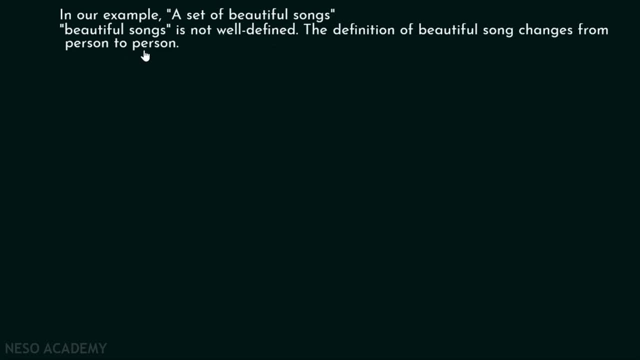 you. The definition of beautiful song changes from person to person. Beautiful songs is not actually well-defined. Okay, Let me tell you how Mark says that a song is beautiful when it is meaningful. So he is my friend, Mark, and he says that a song is beautiful when it is meaningful. 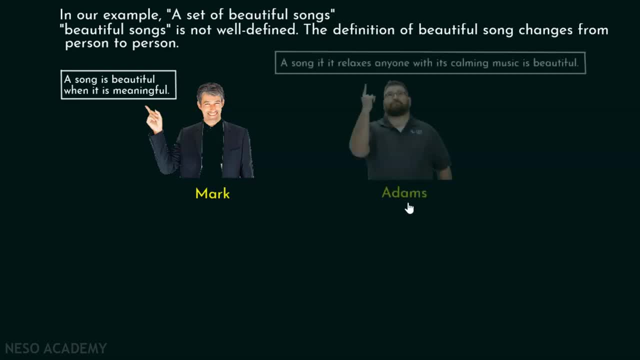 On the other hand, Adam says a song, if it relaxes anyone with its calming music, is beautiful. Now Adam is actually has his own perspective. A song, if it relaxes anyone with its calming music, is actually beautiful. You can see over here that these two people have different opinions and they 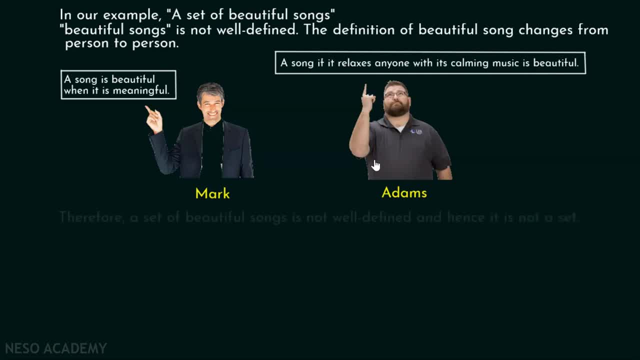 have their own preferences. Therefore, a set of beautiful songs is not well-defined, Isn't that so? Here it is clear that beautiful songs is not well-defined because the definition of beautiful song changes from person to person. Therefore, a set of beautiful songs is not well-defined, Isn't that so? 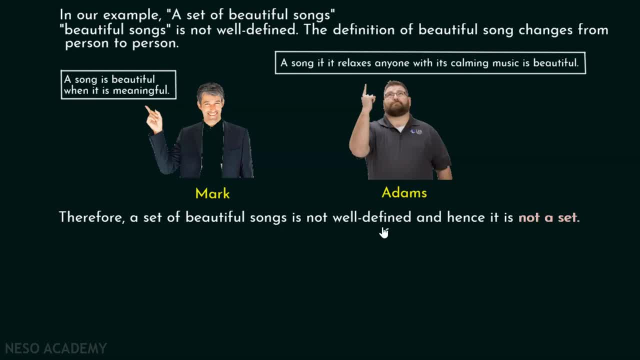 Okay. Therefore, you can say that a set of beautiful songs is not well-defined, Hence it is not a set. A set must be a well-defined collection of objects, Fine, So the term well-defined is very important here. Now here are some more examples. I would like to tell you A collection of great people. 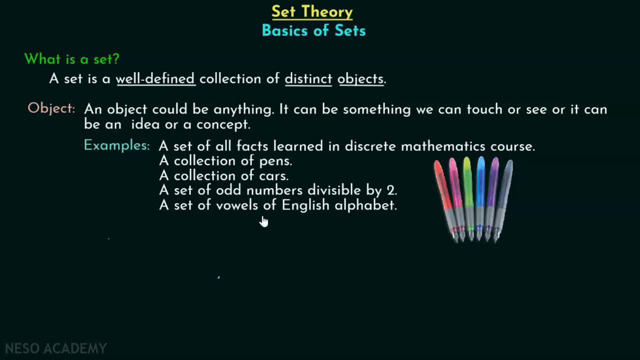 of cars, a set of odd numbers divisible by two, a set of vowels of English alphabet: Pens, cars, odd numbers divisible by two vowels, facts, these are all objects. But what is not a set? A collection of beautiful songs is not set. What, But why? Why? this is not a set. This is where the 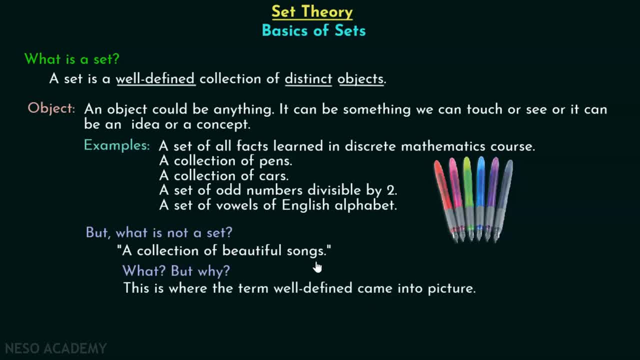 term well-defined came into picture In order to understand this, why this is not a set- we must understand the term well-defined properly. A set is considered to be well-defined if it is possible to establish that any given object belongs to the set. Okay, 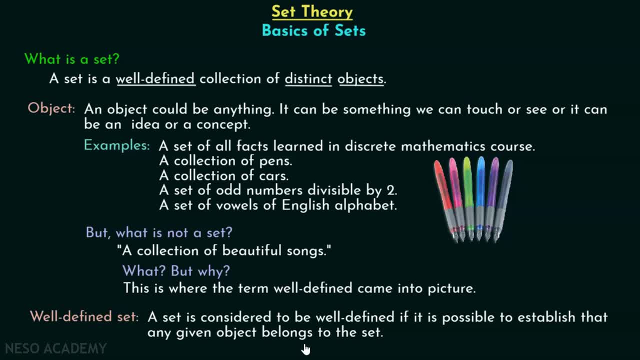 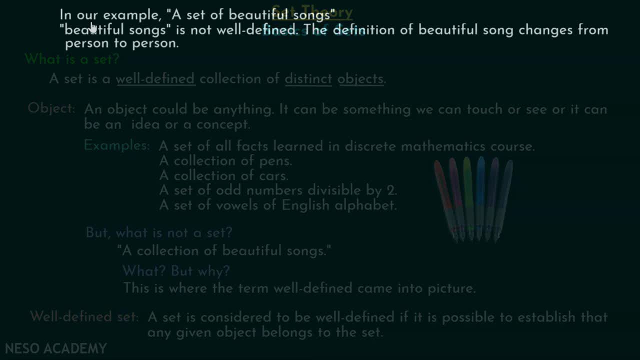 When it is possible to establish this fact, that any given object belongs to the set, then you can say that a set is well-defined. Let's just try to understand this properly with the help of an example. In our example, a set of beautiful songs- beautiful songs- is not well-defined. let me tell. 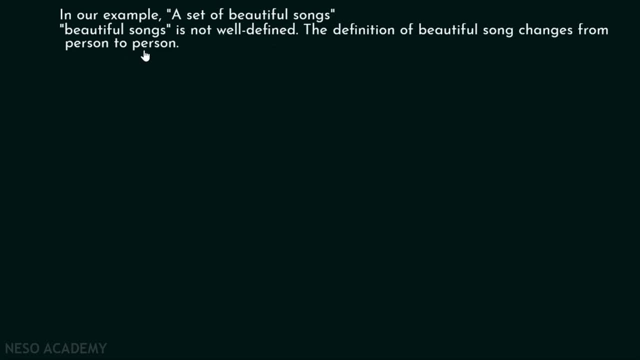 you. The definition of beautiful song changes from person to person. Beautiful songs is not actually well-defined. Okay, Let me tell you how Mark says that a song is beautiful when it is meaningful. So he is my friend, Mark, and he says that a song is beautiful when it is meaningful. 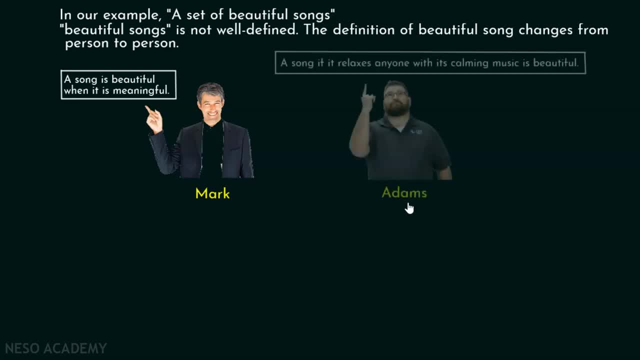 On the other hand, Adam says a song, if it relaxes anyone with its calming music, is beautiful. Now Adam is actually has his own perspective. A song, if it relaxes anyone with its calming music, is actually beautiful. You can see over here that these two people have different opinions and they 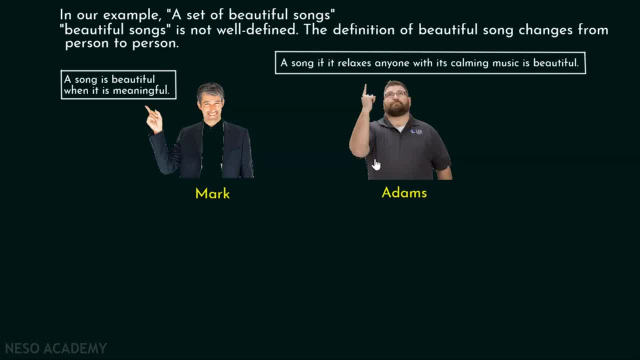 have their own preferences. Therefore, a set of beautiful songs is not well-defined, Isn't that so? Here it is clear that beautiful songs is not well-defined because the definition of beautiful song changes from person to person. Therefore, a set of beautiful songs is not well-defined, Isn't that so? 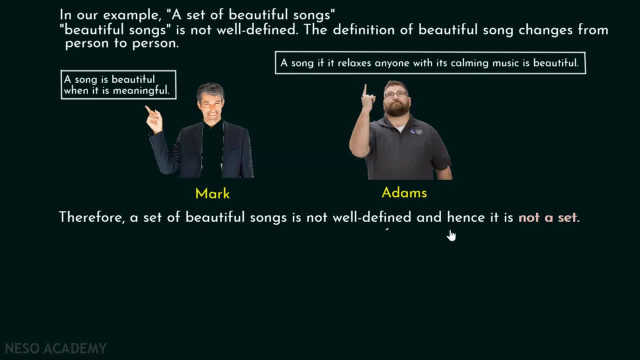 You can say that a set of beautiful songs is not well-defined, Hence it is not a set. A set must be a well-defined collection of objects, Fine, So the term well-defined is very important here. Now here are some more examples. I would like to tell you A collection of great people of the world, A 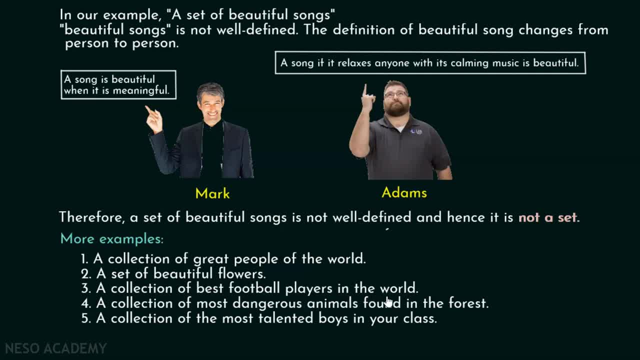 set of beautiful flowers, A collection of best football players in the world. A collection of most dangerous animals found in the forest. A collection of the most talented boys in your class. These are the examples of not a set Fine. After understanding the meaning of well-defined as well as an object. now we'll try to understand. 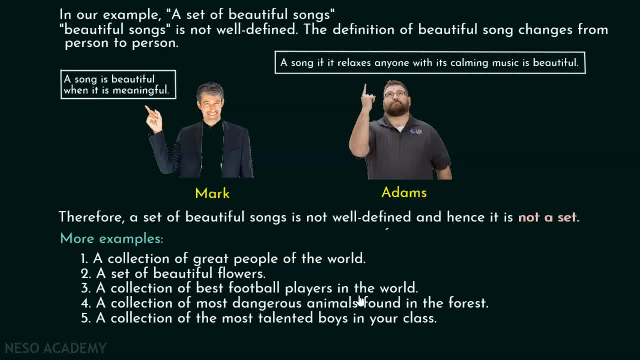 of the world, A set of beautiful flowers, A collection of best football players in the world, A collection of most dangerous animals found in the forest, A collection of the most talented boys in your class. These are the examples of not a set Fine. 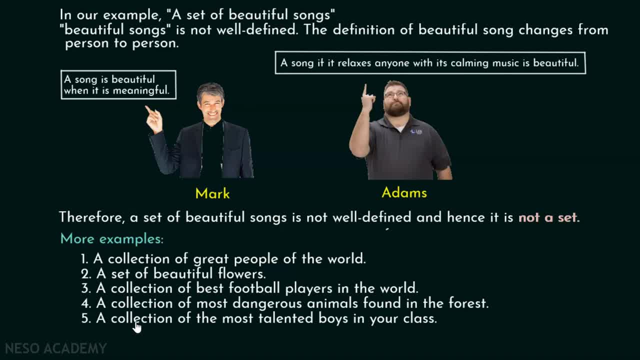 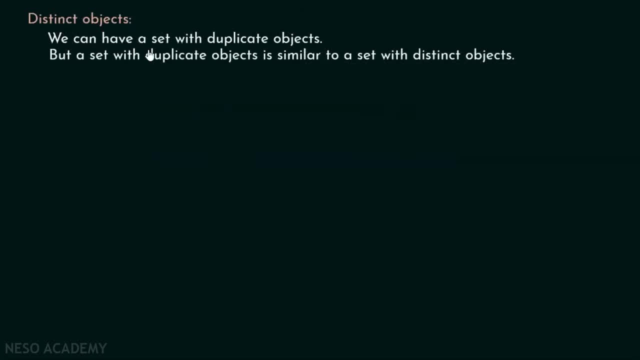 After understanding the meaning of well defined, as well as an object, now we will try to understand the meaning of distinct objects. Fine, What are distinct objects? We can have a set with duplicate objects. let me tell you. But a set with duplicate objects is similar to a set with distinct objects. 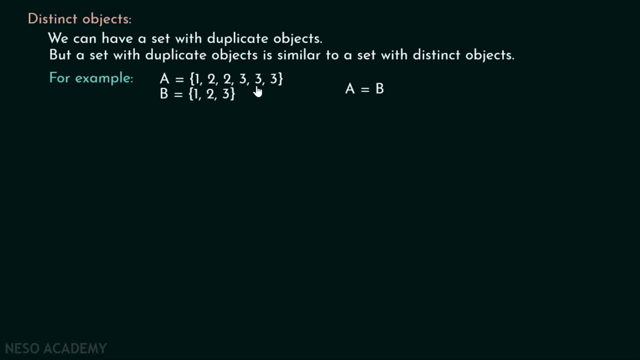 For example, we can have a set like this: A equal to 1,, 2,, 2,, 3,, 3,, 3, and we can have a set like this: B equal to 1,, 2, 3.. Let me tell you that there is no difference between these two sets. They are actually equal. 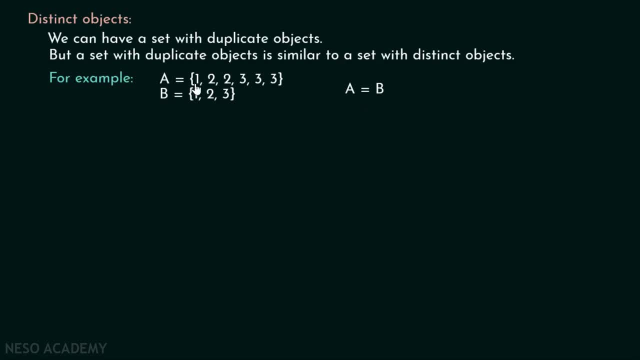 A is actually equal to B, Even though you can clearly see that A has total six elements and B has three elements. But eventually A is equal to B. Actually, in a set, these duplicate objects get eliminated and we end up with a set similar to this set: 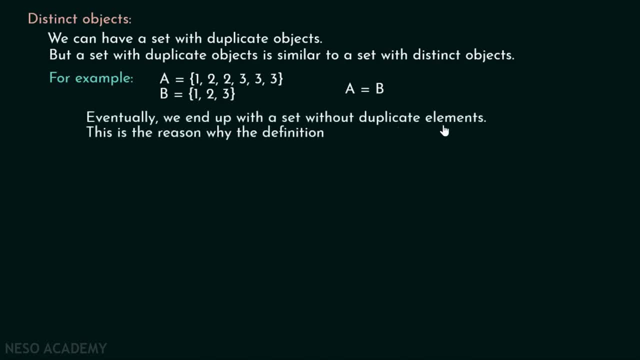 Okay, eventually we end up with a set without duplicate elements. Here you can see that A is equal to B, So it is clear that writing duplicate elements is actually redundant. So it is clear that a set with duplicate objects is actually similar to a set with distinct objects. 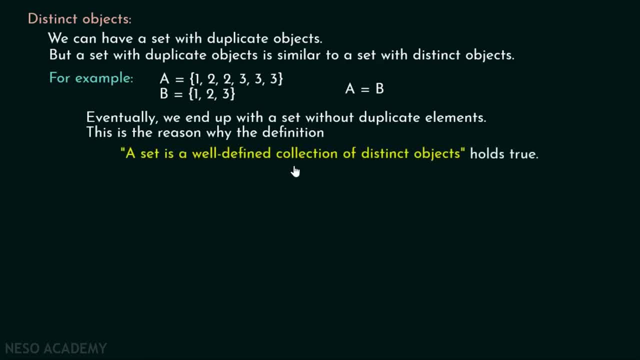 This is the reason why the definition holds true. A set is a well-defined collection of distinct objects. Okay, now you have understood the term set. A set is a well-defined collection. It must be well-defined, fine, And apart from this, there must be distinct objects within it. 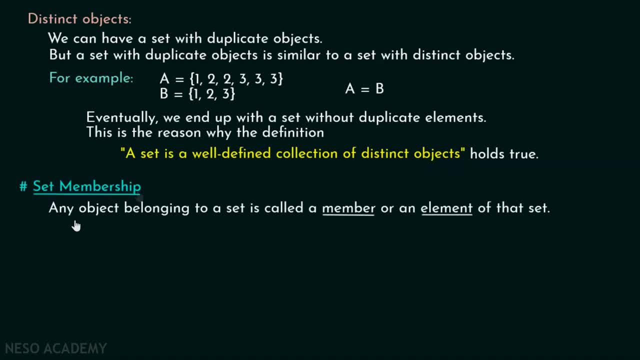 Now let's just try to understand the meaning of set membership. Any object belonging to a set is called a member or an element of that set. So if we say an object and if it belongs to a set, then we can say that that particular object is actually a member or element of that set. 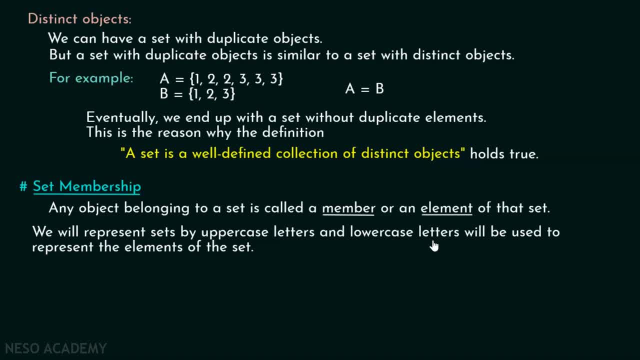 Fine, we will represent sets by uppercase letters, And lowercase letters will be used to represent the elements of the set. From now on, it is very important for us to represent the sets by uppercase letters and we will represent the elements of any set by lowercase letters. 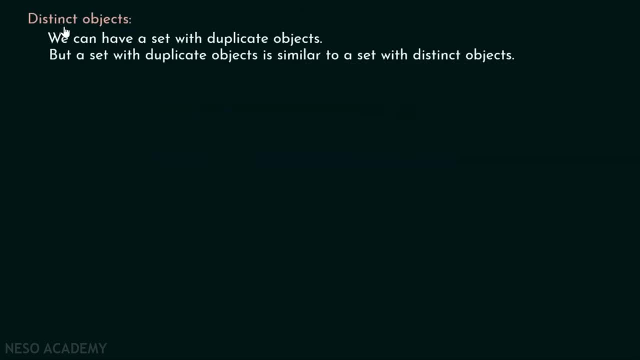 the meaning of distinct objects. Fine, What are distinct objects? We can have a set with duplicate objects. let me tell you. But a set with duplicate objects is similar to a set with distinct objects. For example, we can have a set like this: A equal to one, two, two, three, three, three, And we can 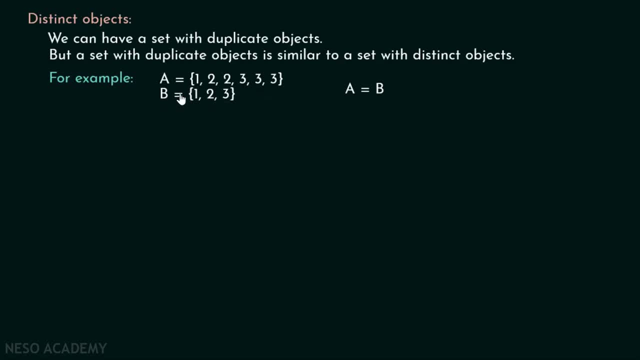 have a set like this: B equal to one, two, three. Let me tell you that there is no difference between these two sets. They are actually equal. A is actually equal to B, Even though you can clearly see that A has total six elements and B has three elements. But eventually A is. 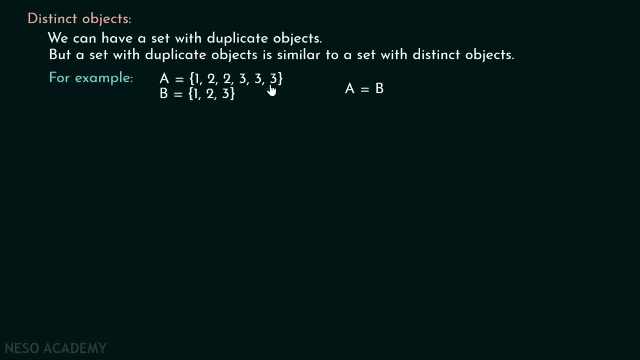 equal to B. Actually, in a set, these duplicate objects get eliminated and we end up with a set similar to this set. Okay, Eventually we end up with a set without duplicate elements. Here you can see that A is equal to B, So it is clear that writing duplicate elements is actually. 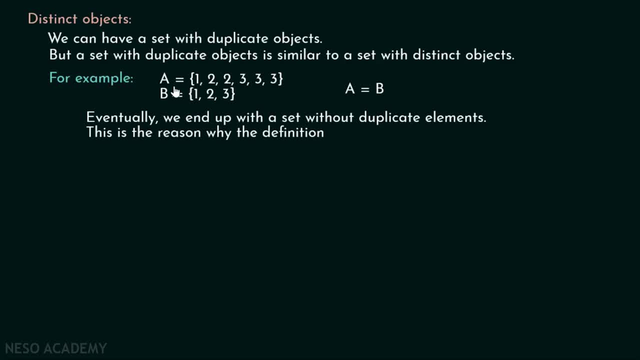 redundant. So it is clear that a set with duplicate objects is actually similar to a set with distinct objects. This is the reason why the definition holds true. A set is a well-defined collection of distinct objects. Okay, Now you have understood the term set. A set is a. 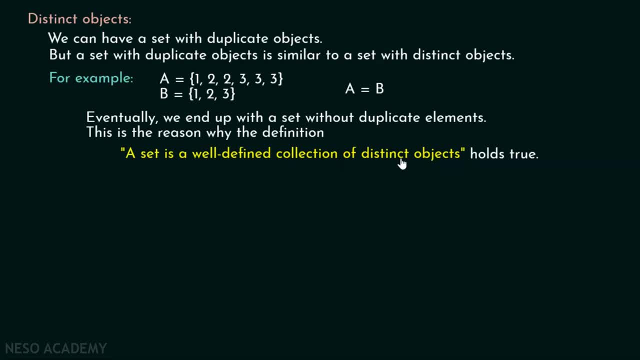 well-defined collection. It must be well-defined, Fine, And apart from this, there must be distinct objects within it. Now let's just try to understand the meaning of set membership. Any object belonging to a set is called a member or an element of that set. So if we say an object, 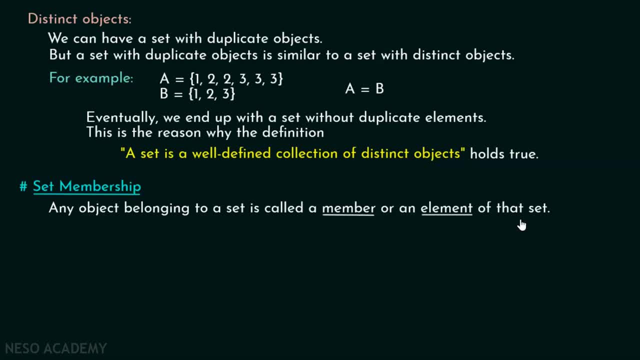 and if it belongs to a set, then we can say that that particular object is actually a member or element of that set. Fine, We will represent sets by uppercase letters, and lowercase letters will be used to represent the elements of the set From now on. it is very important for us to 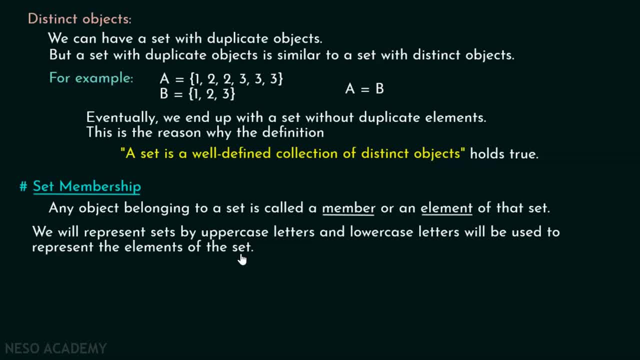 represent the sets by uppercase letters and we will represent the elements of any set by lowercase letters. If A is an element of set A, then we can say that A belongs to A. This symbol is actually called belongs to symbol. Fine, So A belongs to A. or we can say A is in A If 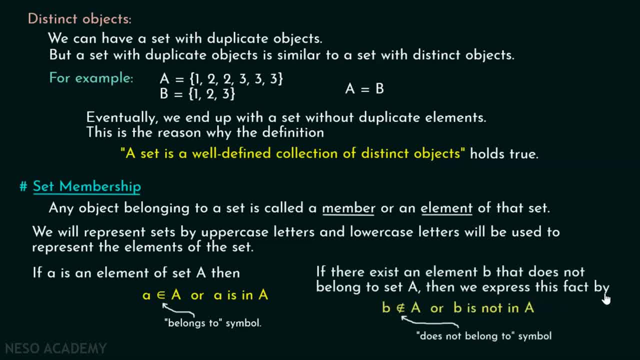 there exists an element B that does not belong to A, then we express this fact by: B does not belong to A. The symbol is called: does not belong to B, belong to symbol. So here B does not belong to A, because we are saying that B is not in A.